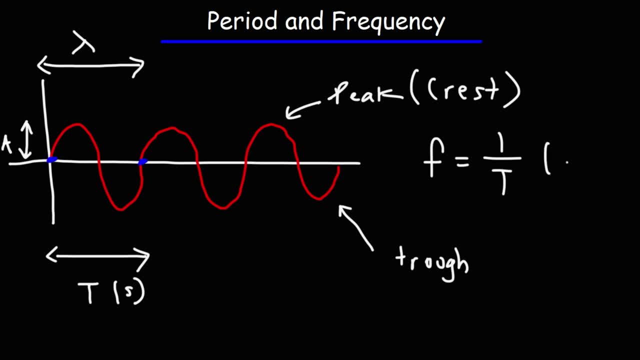 the second, and the standard unit for frequency is Hertz. so one hurt or one Hertz is one second to the minus one, it's 1 over s. now the speed of the wave is basically the wavelength divided by the period, so you can see this as wavelength times 1 over the period, and 1 over the period is the. 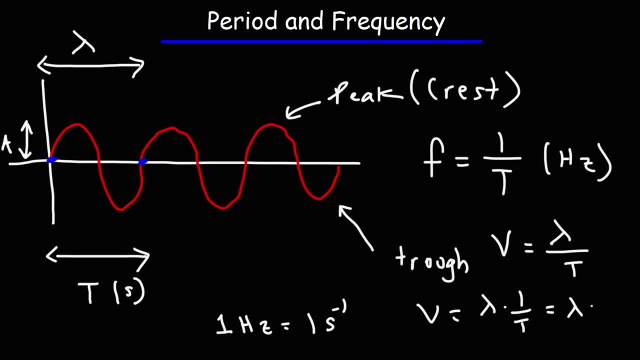 frequency. so the velocity of the wave, or the speed of the wave, is the wavelength times the frequency. so these are two important equations that you want to remember. frequency is 1 over the period and the wavelength times the frequency is equal to the velocity. now, if you want to calculate, 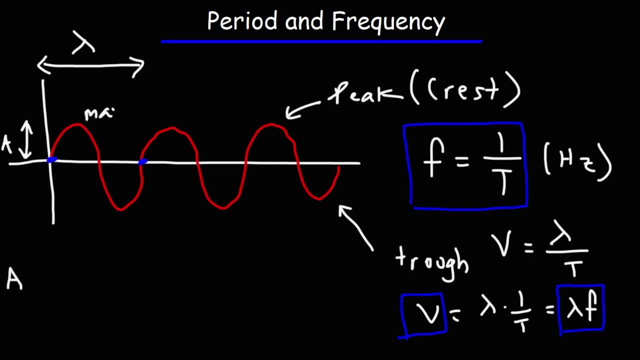 the amplitude, and if you know the maximum value and the minimum value, the amplitude is basically just one half of that. it's the max minus the minimum value, which gives it a range divided by 2. so that's how you can calculate the amplitude of a wave. so now let's 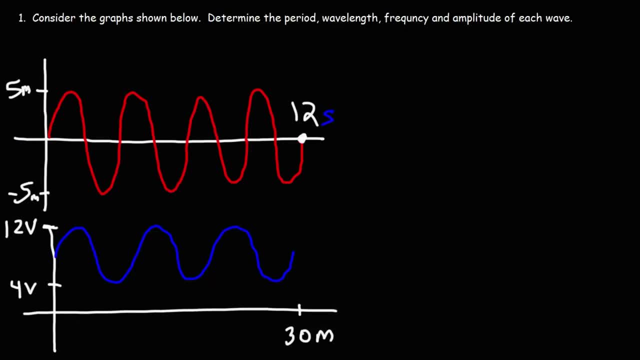 work on some problems. consider: the graphs shown below. determine the period, wavelength, frequency and amplitude of each wave. so let's start with the period. the period is the time it takes to complete one cycle. you can also calculate it by taking the total time, dividing it by the total number of cycles. so how many cycles do we have in the red? 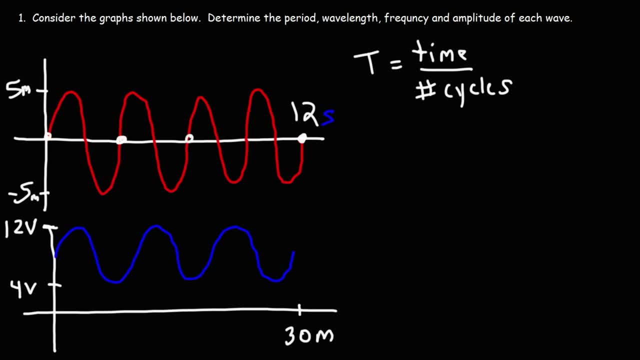 wave starting from here. this is the first cycle, second cycle, the third one and this makes the fourth the fourth cycle. so in 12 seconds this wave has undergone four cycles. divided by four is three. that means it takes three seconds for this wave to complete one cycle. 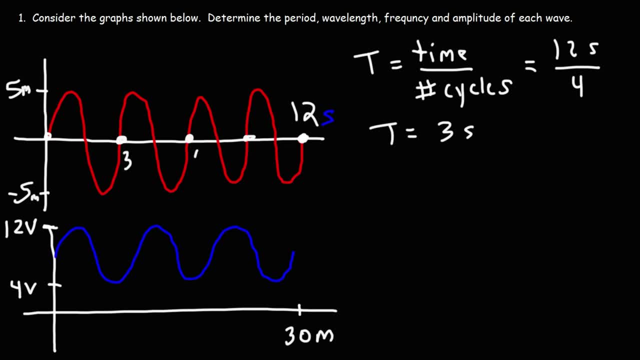 so this is three, this is six, this is nine and that's twelve. so that's the period, the time it takes to complete a single cycle. now, the frequency is one over the period, so that's one over three seconds, which is approximately 0.33 Hertz. the period I mean, the frequency, is also the reciprocal of this formula. the frequency 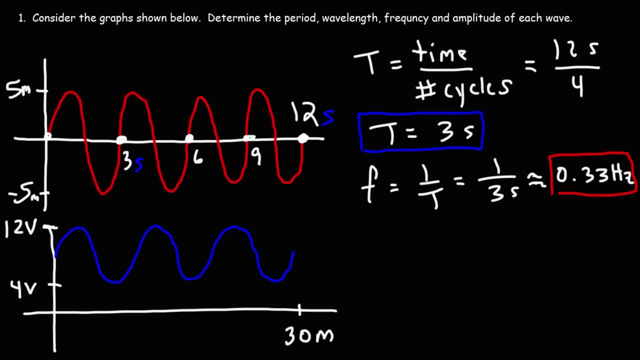 is the number of cycles divided by the time, or the number of cycles that a wave goes through every second. now let's talk about the amplitude. we can't find a wavelength for this particular wave because we just don't have the information. in this particular wave, the red wave, we have time on the. 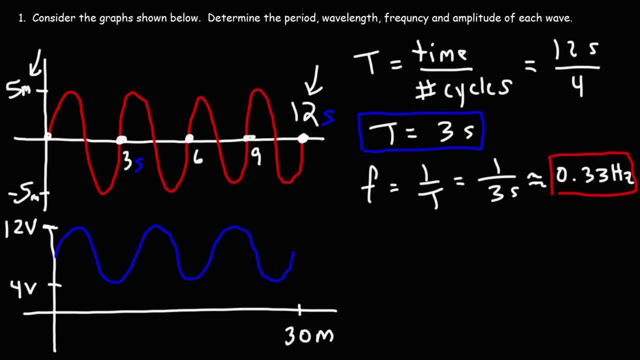 x-axis meters or displacement on the y-axis. when you see units like meters, feet on the y-axis, that means that the wave it's a displacement wave. you're measuring displacement with time, so we can't find the wavelength for that, but we can find the amplitude. the amplitude is basically this: 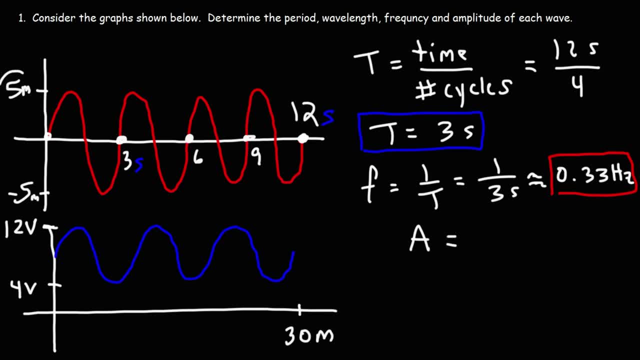 number five. keep in mind it's the top number minus the bottom number divided by 2, so it's 5 minus negative five divided by 2, so this becomes 5 plus 5, which is 10. 10 over two is five, in this case the displacement. 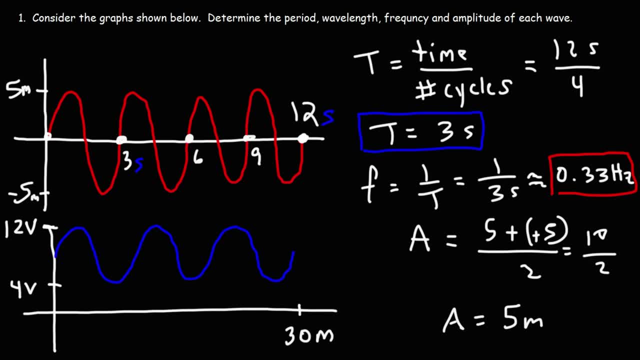 amplitude is five meters. that's all we could do for the first wave. now for the second wave, the blue wave. notice that we have meters on the x-axis. that's going to help us to find the wavelength wavelength. Now we don't have time or seconds in the x-axis, so we can't find. 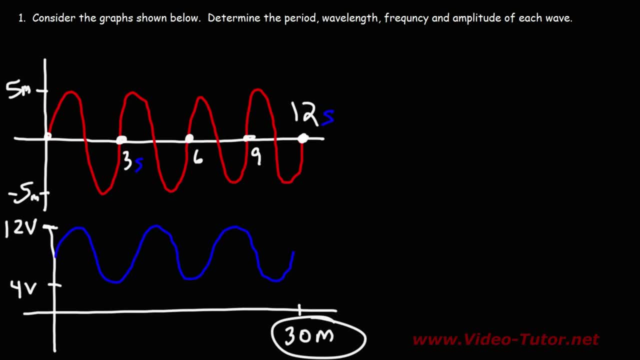 the period or frequency for the blue wave, but we can find the wavelength. So this is one cycle, two cycles, three cycles. So 30 meters divided by three cycles, that means that we have 10 meters per cycle And that's the wavelength. the 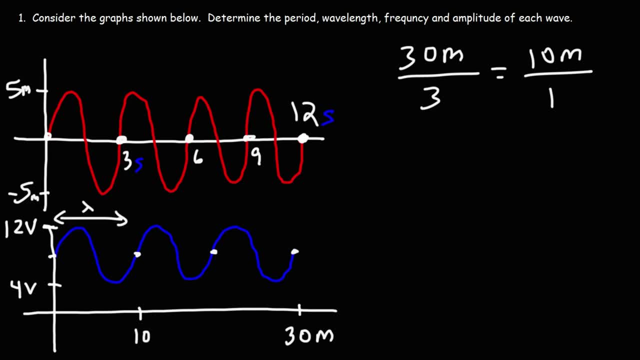 distance between cycles. So the wavelength in this example is 10 meters. Now we can calculate the amplitude for this wave. I probably should have designed the problem better, rather than saying: you know, determine all four of these for each wave. Now, on the y-axis, we have voltage. The max voltage is 12. 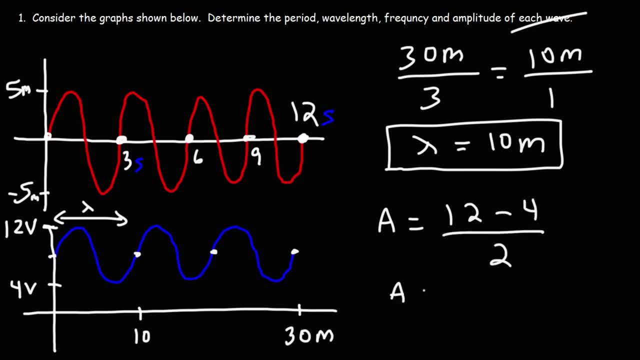 and the amplitude is 10.. So we can calculate the amplitude for each wave. Now, on the y-axis, we have voltage. The max voltage is 12, the minimum voltage is 4, and we're gonna divide that by 2.. 12 minus 4 is 8.. 8. 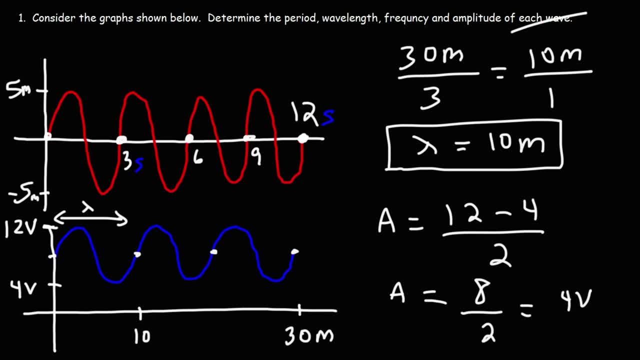 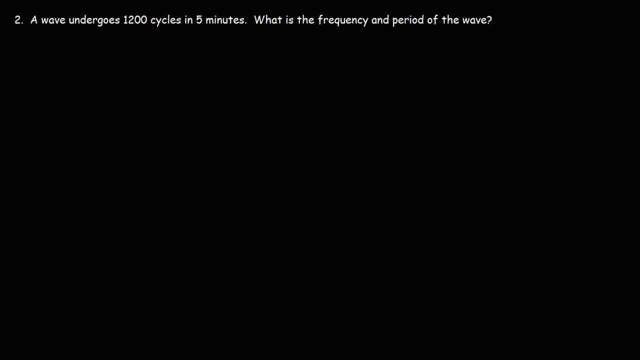 divided by 2 is 4.. So the amplitude for the blue wave is 4 volts. So now you know how to calculate the period, wavelength, frequency and amplitude of a wave. Let's move on to this problem. A wave undergoes 1,200 cycles in 5 minutes. What is the? 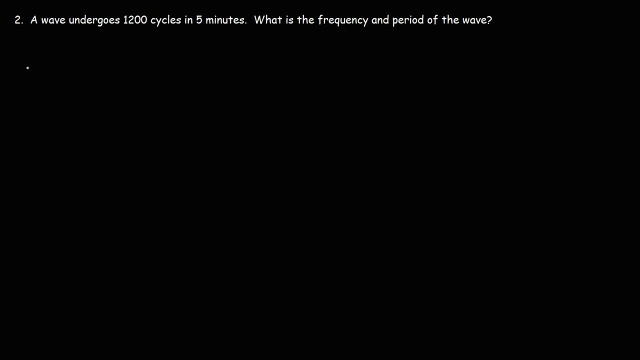 frequency and period of the wave. We could use this formula to calculate the frequency. The frequency is the number of cycles that occur every second. So if we take the total number of cycles and divide it by the time, we can get the frequency. Now we need the time. 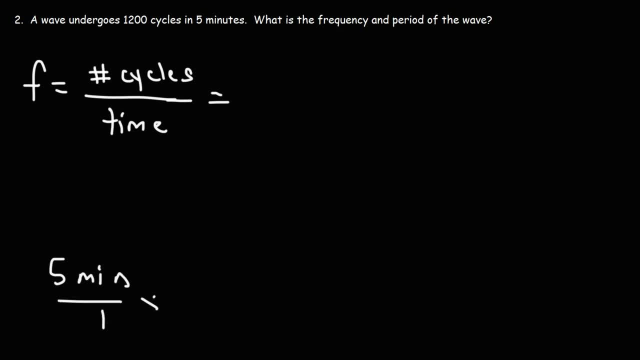 in seconds. so we need to convert minutes into seconds And keep in mind there's 60 seconds in every minute. So multiplying 5 by 60 will give us the time in seconds. 5 times 6 is 30, add a zero, we get 300 seconds. So we have twelve hundred cycles. 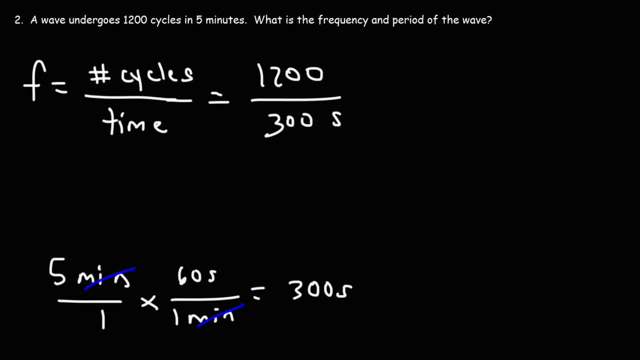 occurring in 300 seconds. So let's cancel two zeros, So becomes 12 over 3.. So there's four cycles occurring per second. So this means that the frequency is 4 Hertz. It's the number of cycles that the wave goes through per second. 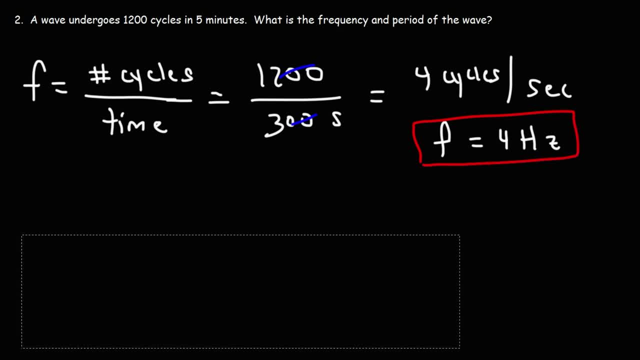 That's the number of cycles that the wave goes through per second. That's the number of cycles that the wave goes through per second that we have the frequency, we can calculate the period. so, remember, the frequency is 1 over the period. the period is also 1 over the frequency. so 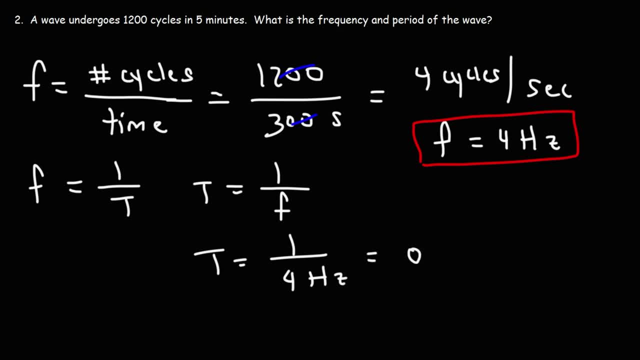 1 over 4 Hertz 1 over 4 is 0.25, so this is going to be point 25 seconds. so that's how you can calculate the frequency in the period of this particular wave. now let's move on to number 3. what is the wavelength of a 3? 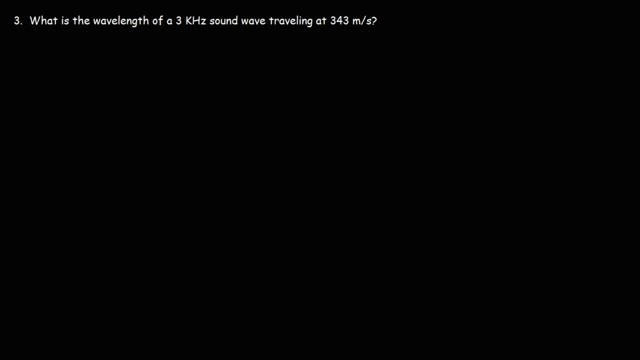 kilohertz sound wave traveling at 343 meters per second. now, if you remember the wavelength, which is represented by the Greek symbol, lambda, wavelength times frequency is equal to the velocity or, in this case, the speed of the wave. we have the speed of the wave, which is 343 meters per second. we know the frequency. 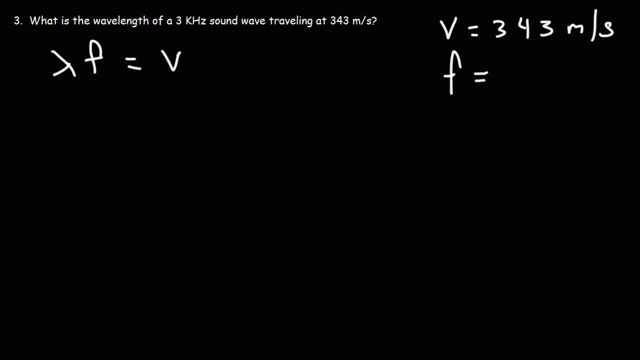 it's 3 kilohertz. K means kilo kilos a thousand, so this is 3000 Hertz. our goal is to calculate the wavelength. so if we divide both sides of the equation by F, we get the wavelength. the wavelength is the speed divided by. 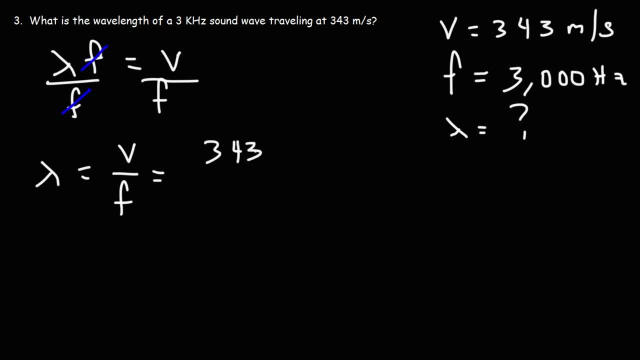 the frequency. the speed is 343 meters per second. the frequency is 3000 Hertz. keep in mind 1 Hertz is 1 over seconds, so the unit seconds will cancel giving us the wavelength in 60. desapare, Emperor. so now let's do the math. so it's going to 343 divided by 3000, and so the 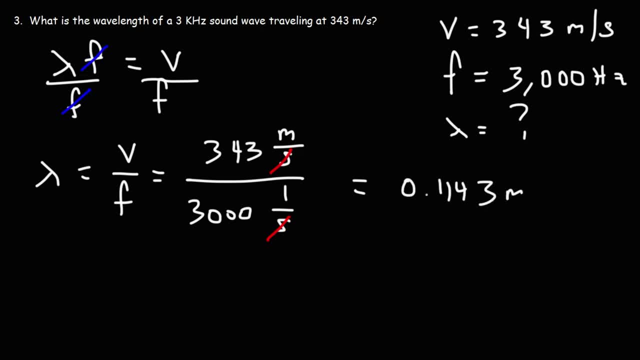 so the wavelength is point 1143 meters. if you multiply that by a hundred, you can convert that to centimeters. so that's eleven point forty three centimeters. so that's how you can find the wavelength, given the frequency and the speed of the wave. 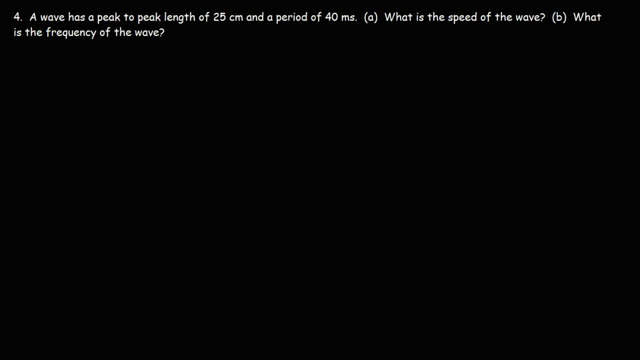 4.8 Fronteras. A wave has a peak-to-peak length of 25 centimeters and a period of 40 milliseconds. What is the speed of the wave? So let's draw a wave. So this is one cycle of the wave. 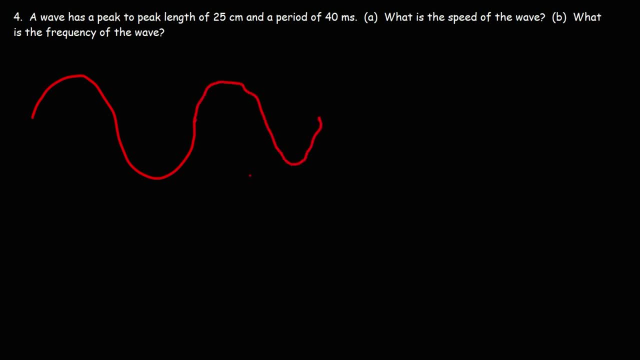 But if we continue it now we have a second cycle- You could find a wavelength between these two points, or from one peak of the wave to the other peak of the wave, So that peak-to-peak distance, that's the wavelength.